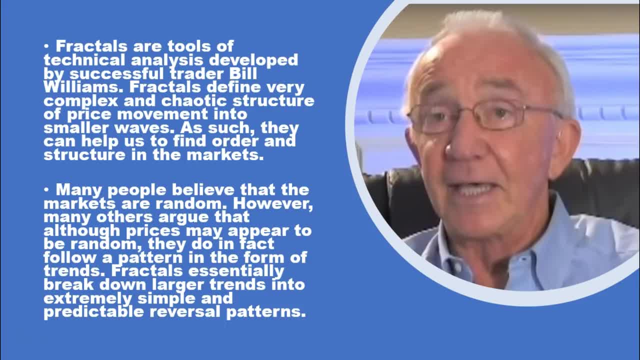 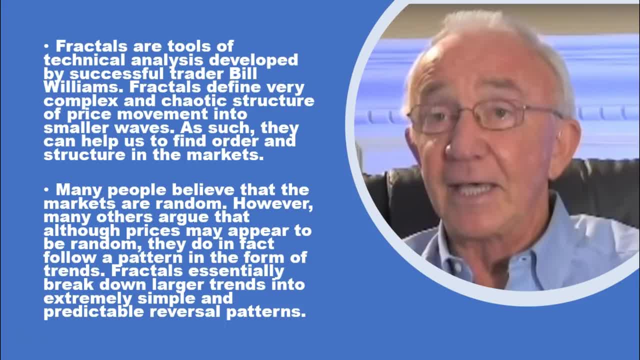 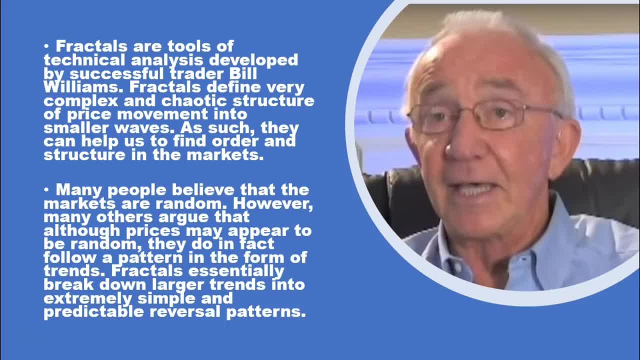 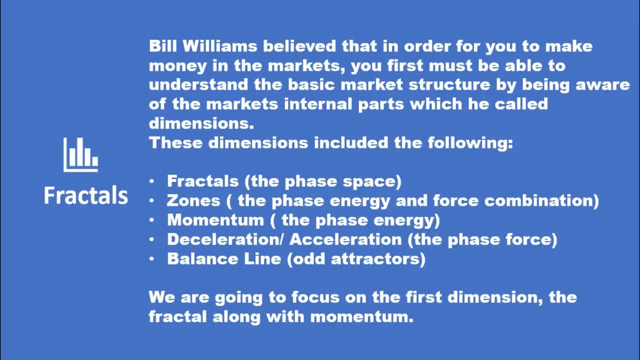 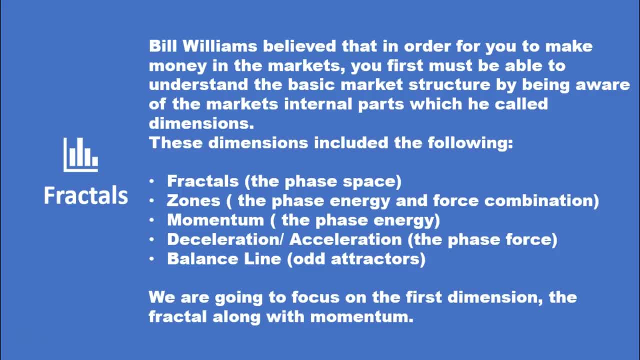 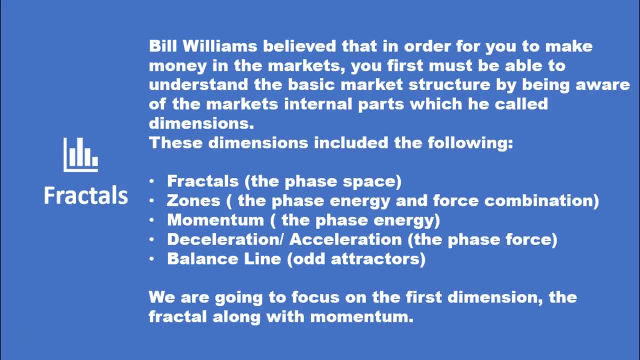 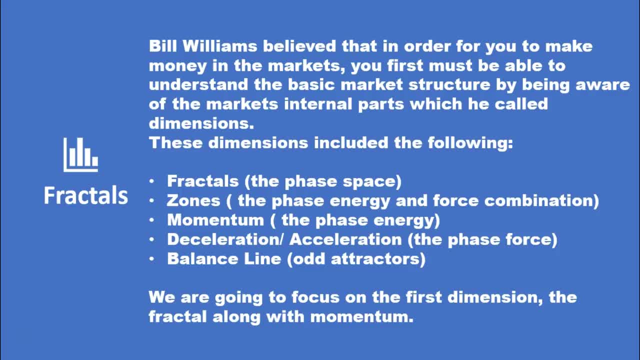 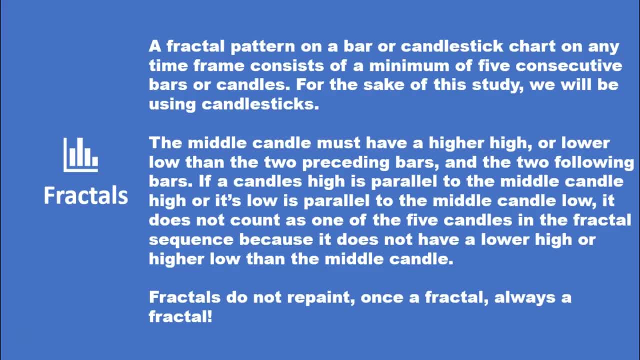 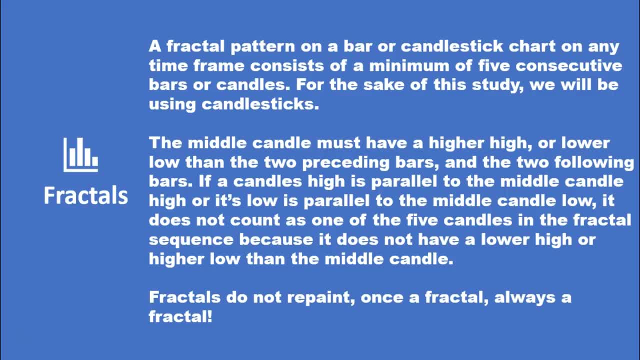 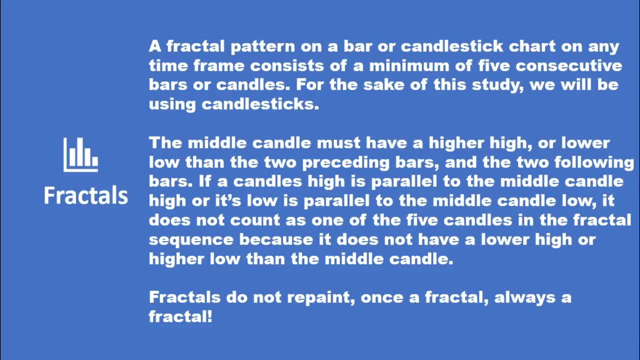 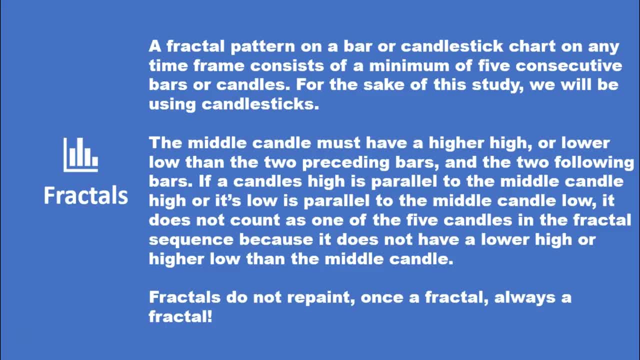 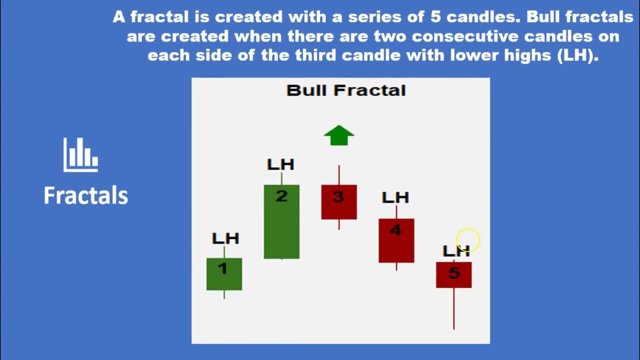 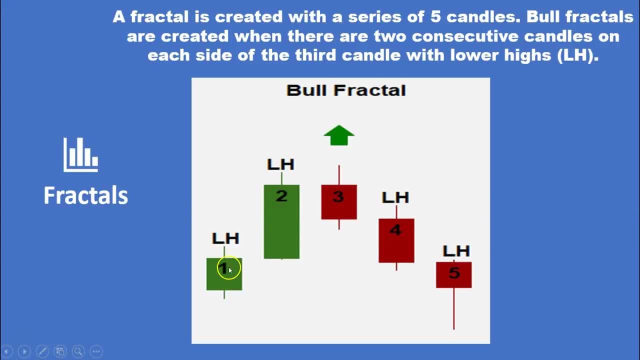 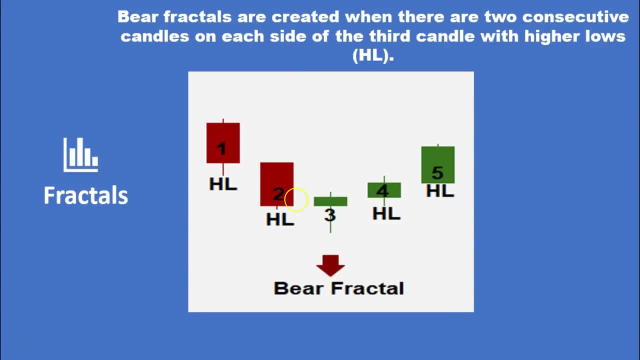 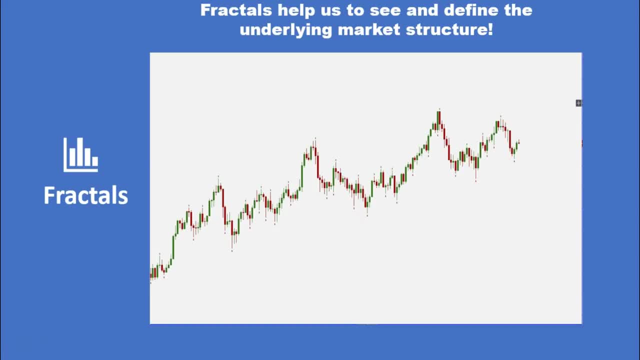 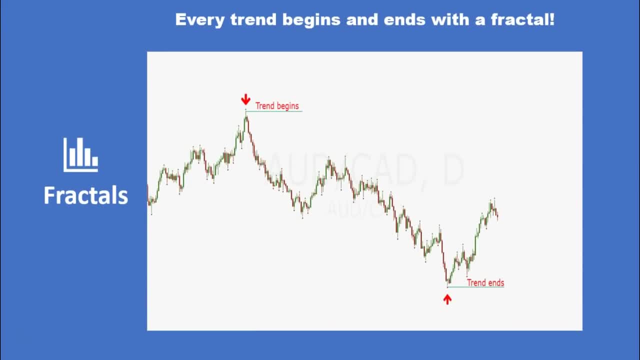 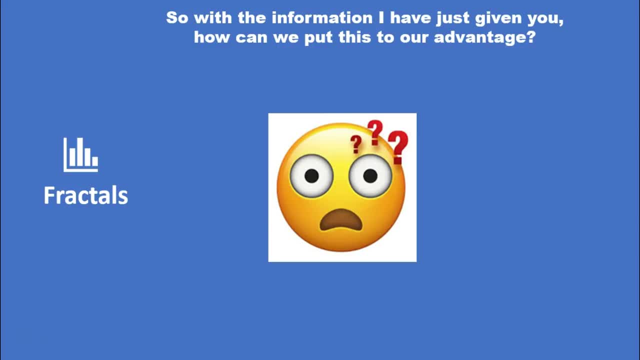 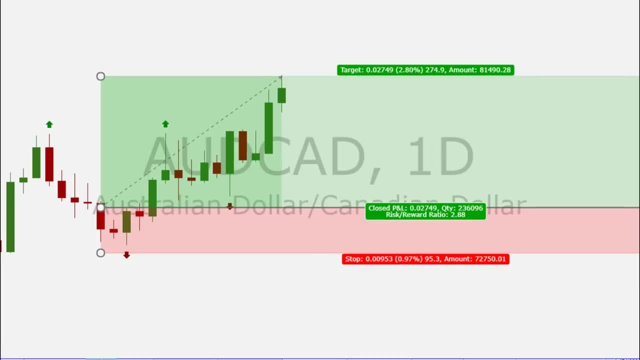 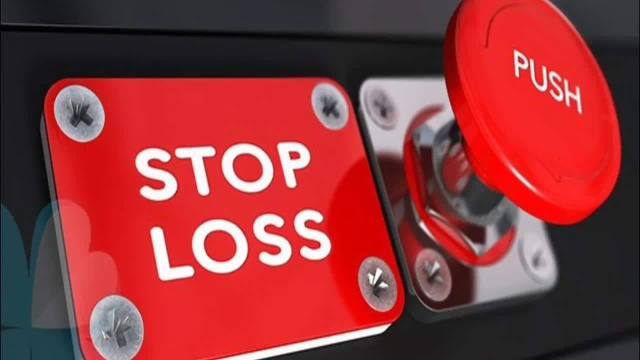 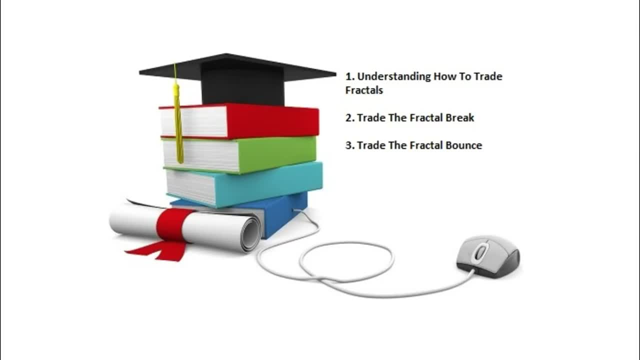 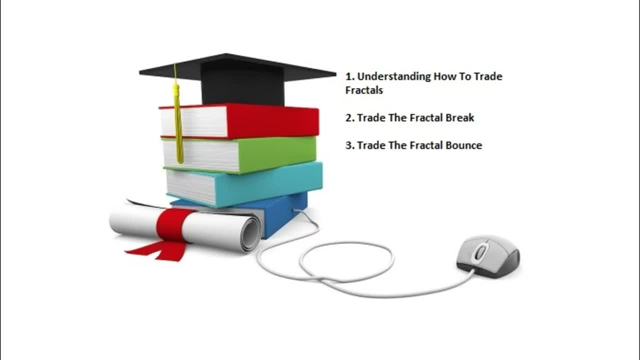 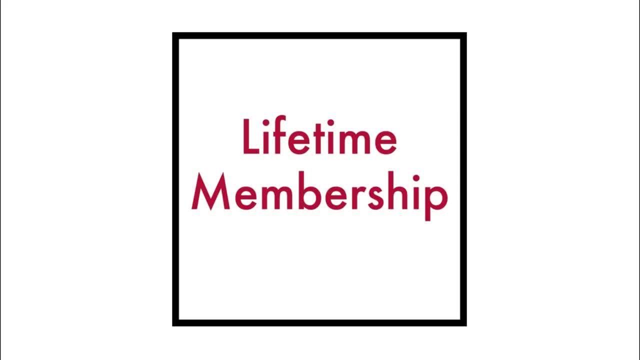 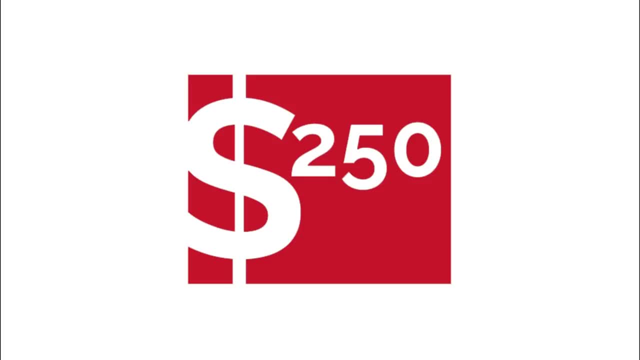 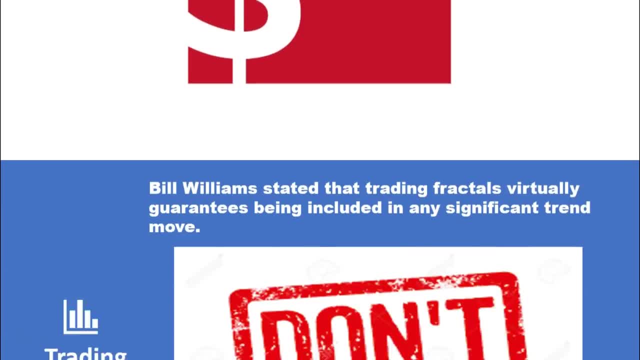 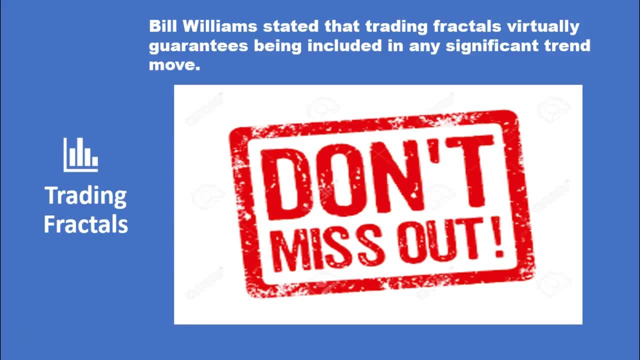 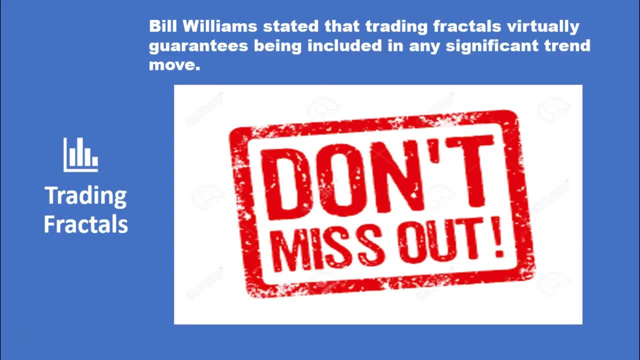 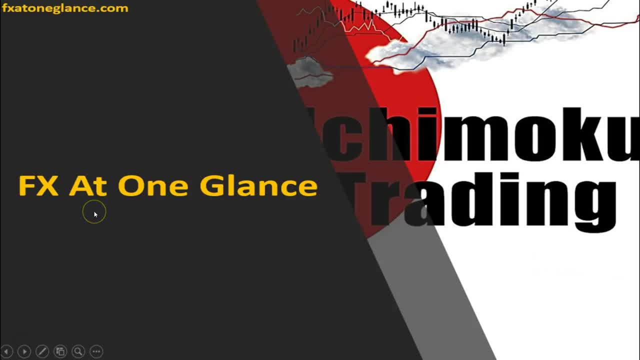 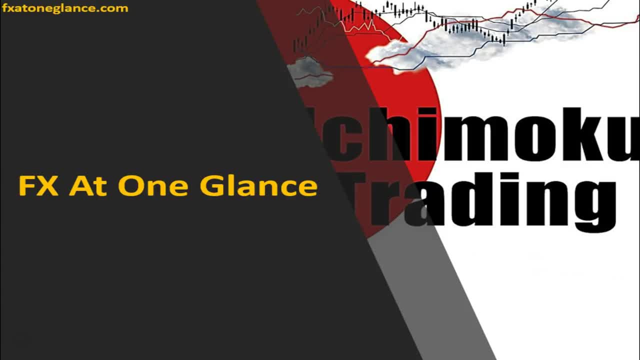 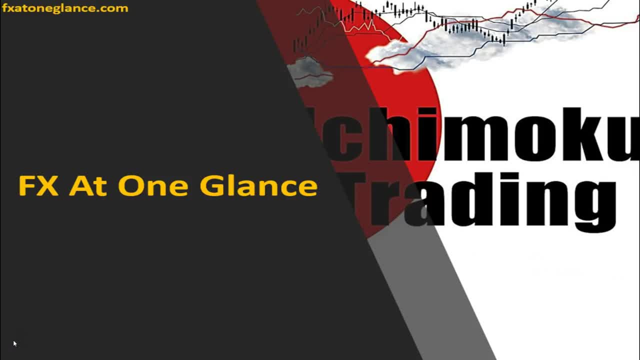 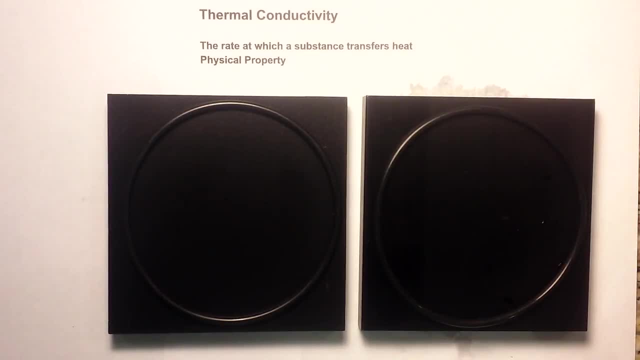 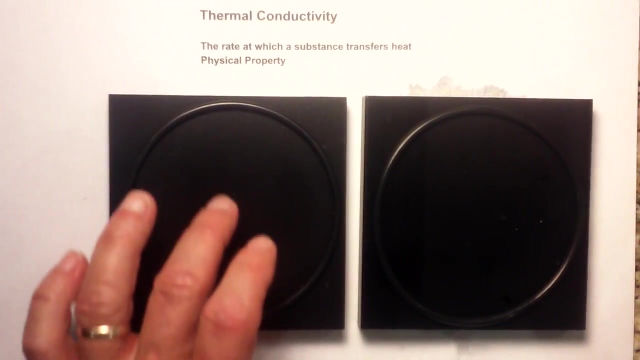 In this video I'd like to talk about thermal conductivity. Thermal conductivity is a physical property and it's the measure of the rate at which a substance transfers heat And the demonstration I have. I have two metal squares. excuse me, not metal squares, but two different.